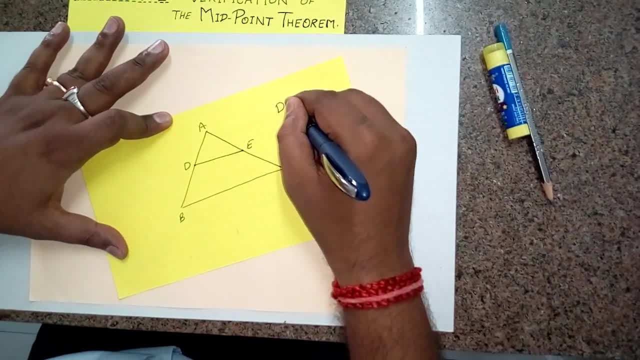 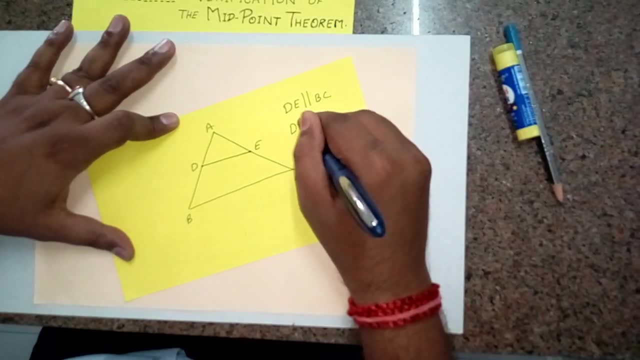 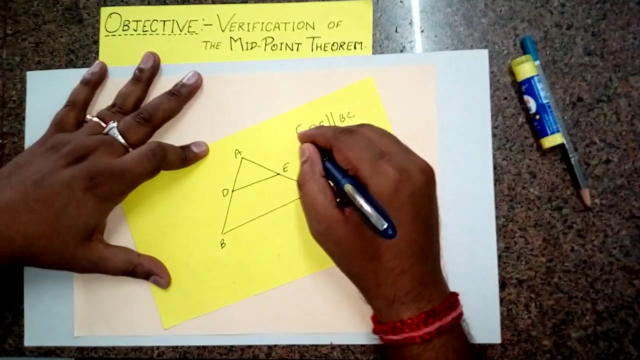 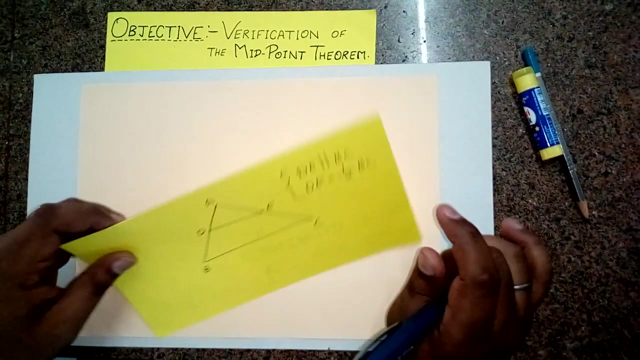 That is, this DE will be parallel to the third side BC And this DE Will be half of the third side BC. This is the theorem. Now we are going to verify these things. That is, this DE will be parallel to BC and DE will be half of BC. by paper folding, cutting and pasting method. 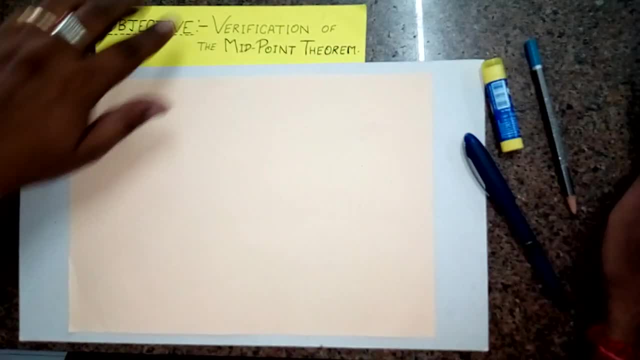 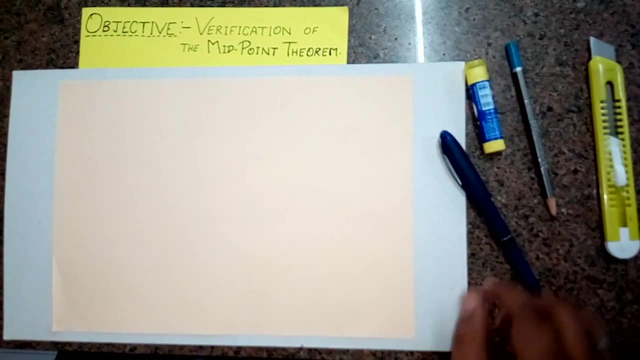 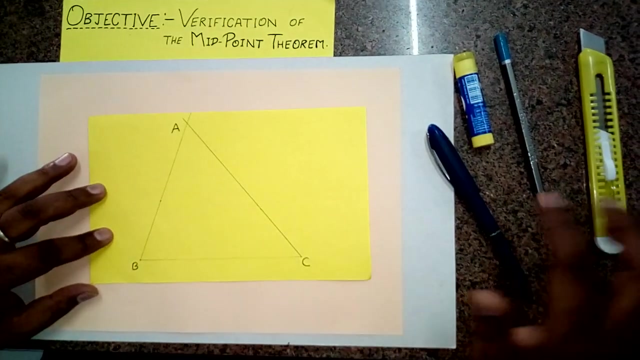 For this we need glow stick, cutter, ruler, pencil, pen and few sheets of paper, Colored paper. you can take any type of colors. Now, first step: Draw a triangle, Any type of triangle, whatever you want. I have taken a scale and triangle AB and C. 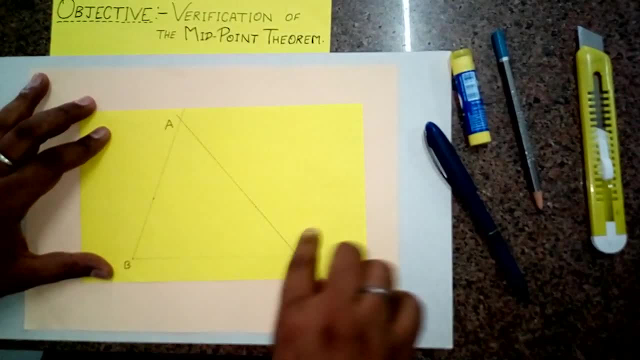 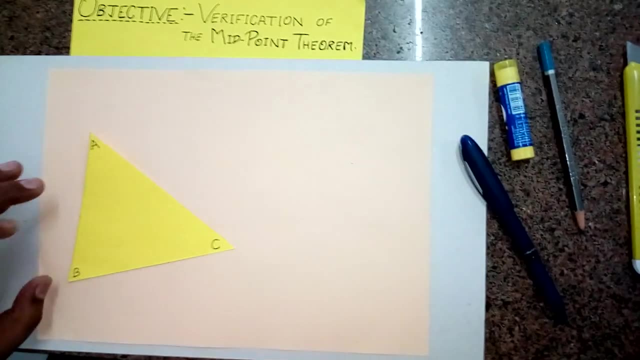 Now, since we have to cut this one, So cut the triangle ABC along its sides. I have already cut it And taken the triangle ABC. Now the theorem was to get the midpoints of the side AB and AC. So first we have to obtain the midpoints. 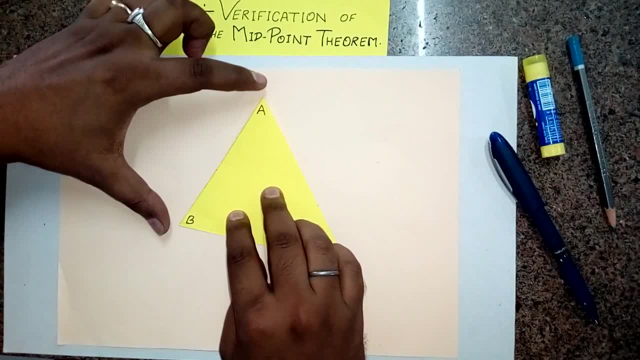 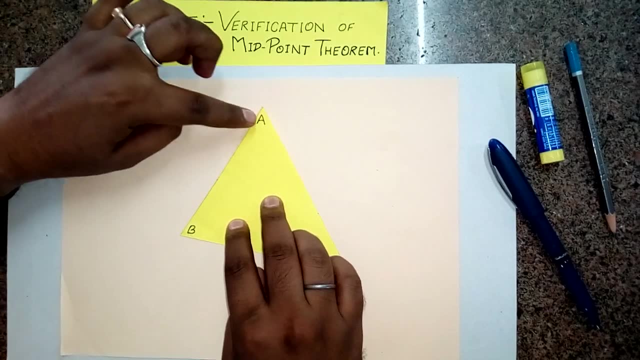 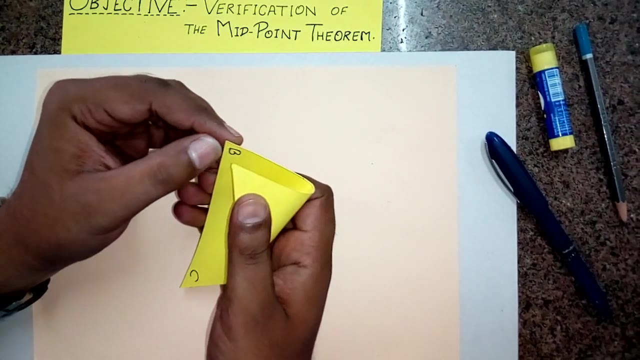 So for this, watch carefully That since we have to obtain the midpoint of AB, So I am folding the side AB So that the point O- Sorry A- Will overlap with the side B. Watch carefully, Point A will overlap with point B. 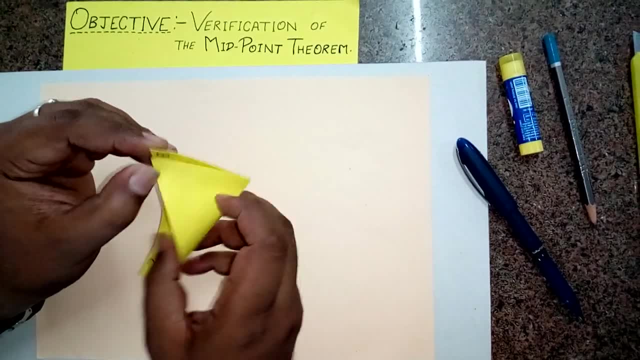 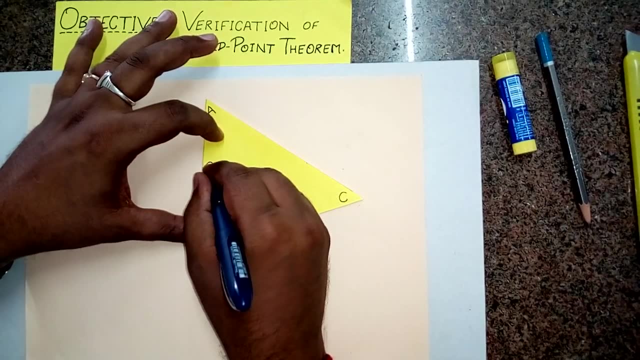 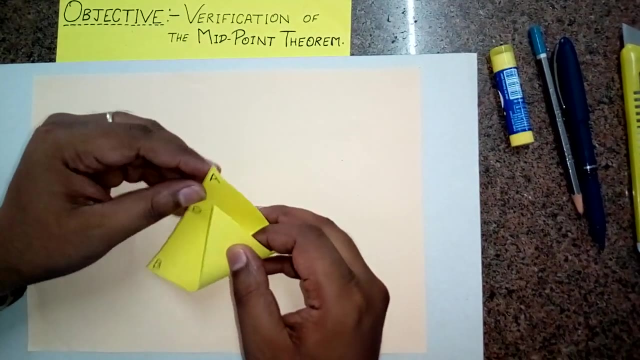 Press it So that you get a firm midpoint. And this is the midpoint, And I am naming it as B. Now, in the same way, we are going to obtain the midpoint of the side AC. So folding So that C will overlap with A. 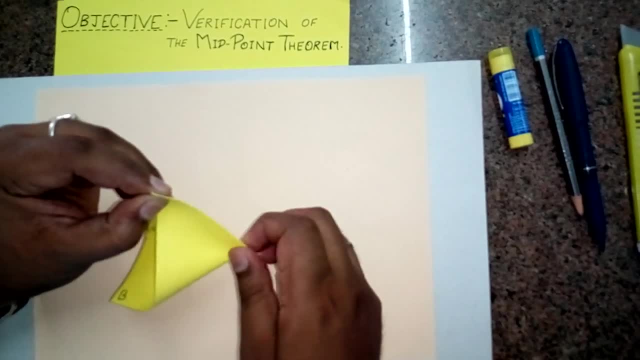 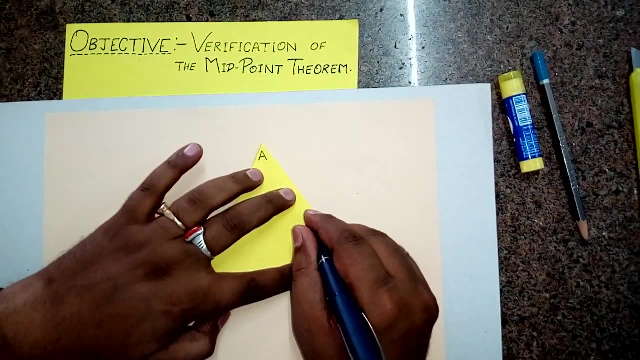 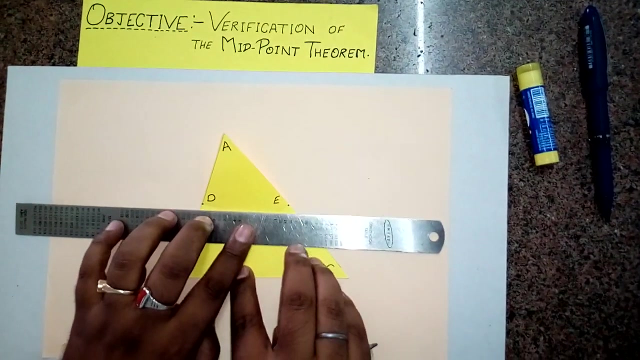 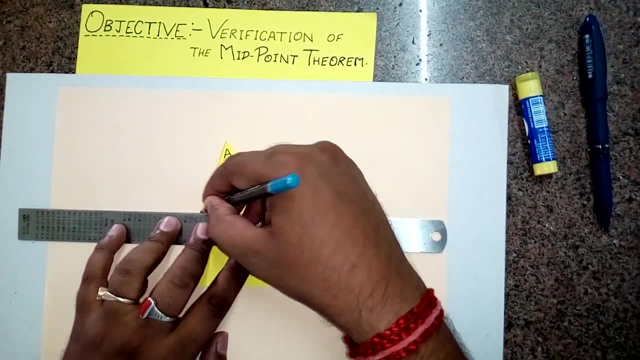 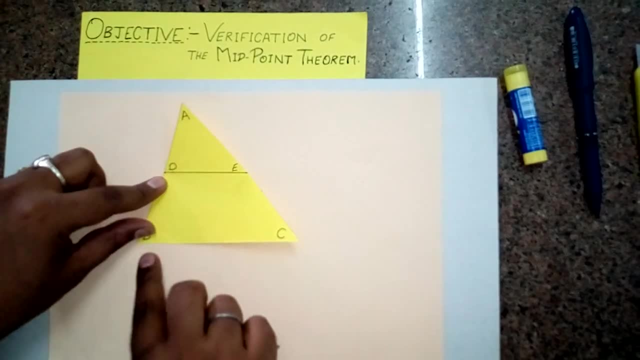 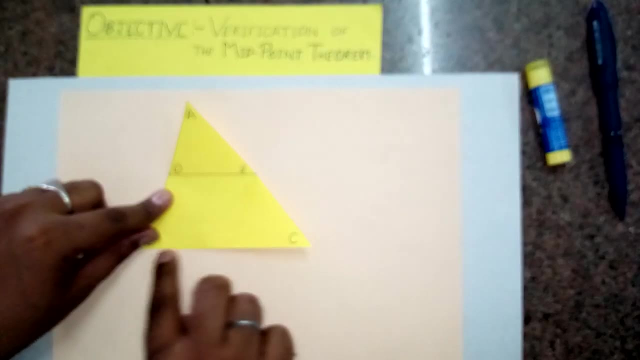 So we have got the line segment DE. Now we are going to prove that this line segment DE will be half of BC and this line segment DE will be parallel to BC. Now, since we have proved that this one is half of BC, so we need the half of BC also. So let me obtain the 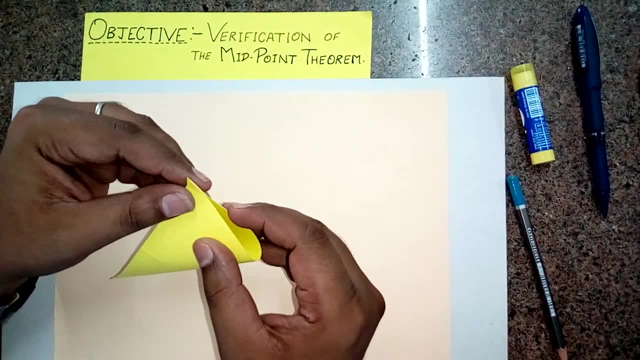 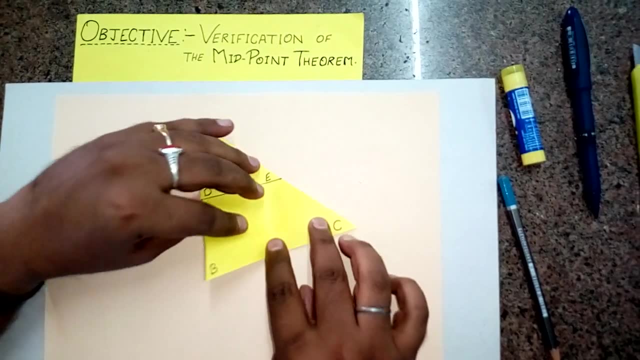 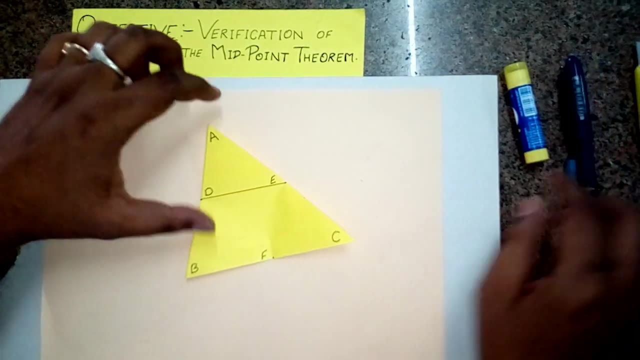 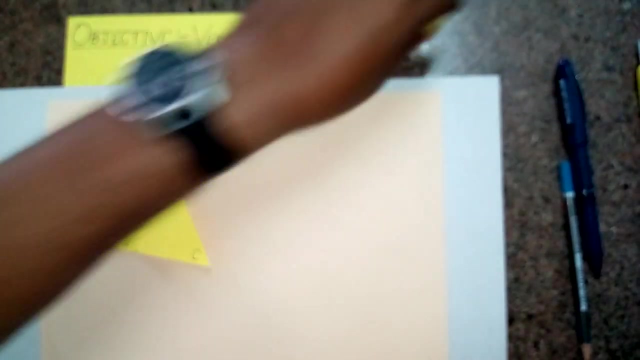 half, that is midpoint of BC. Overlap B with C and fold it to get the midpoint of BC. I am naming it as F. So we have got the triangle, the midpoint and the line segment DE. So next I am going to paste this triangle on this sheet on which I am going to write the observation. 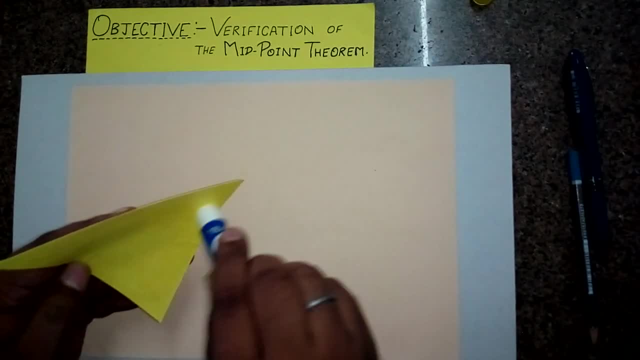 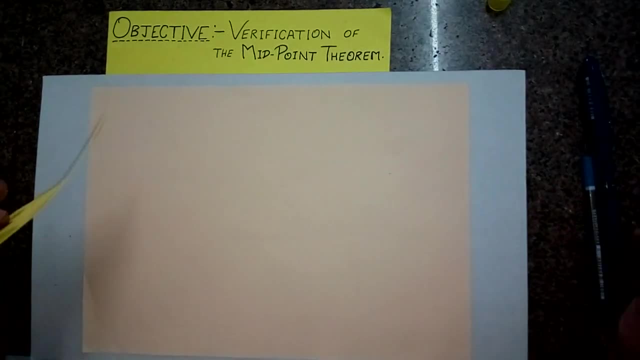 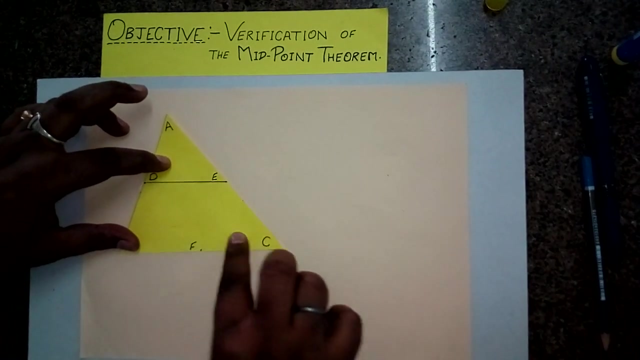 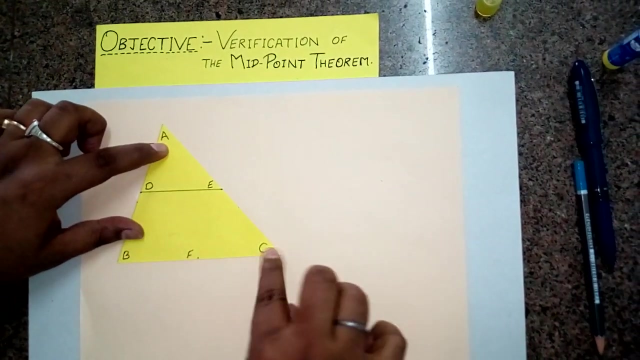 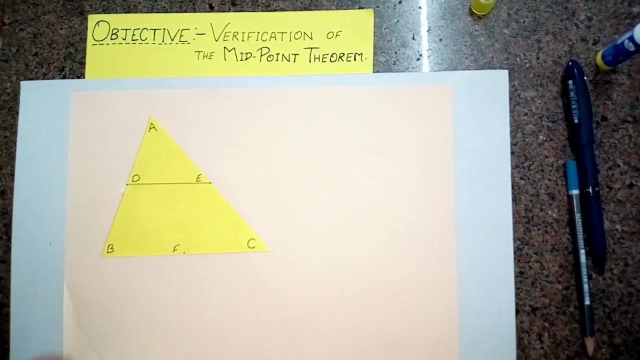 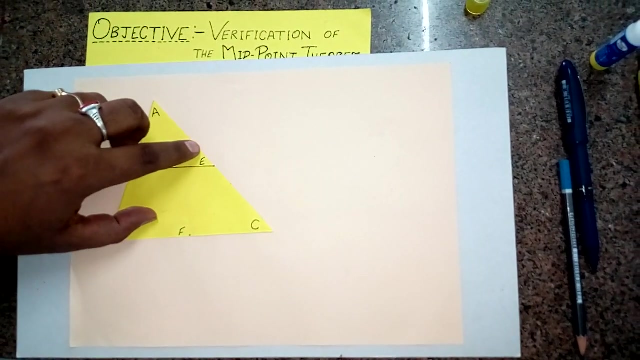 DE. So let me apply some glue over it Now, since we need to prove that these lines are parallel, and we have learnt that two lines are parallel if the corresponding angles are equal. So I am going to prove that this angle, AED will be equal to ACB, So these two angles will. 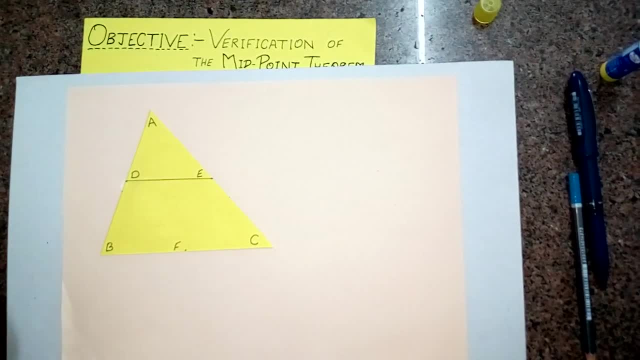 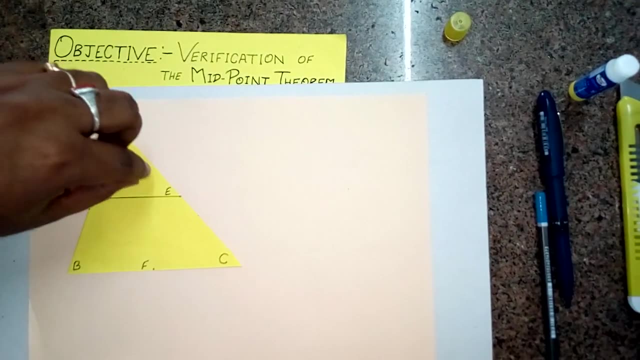 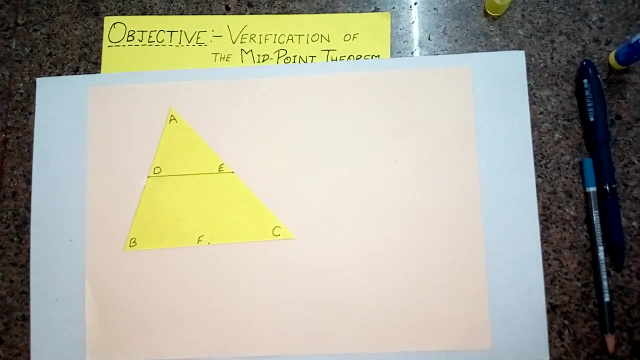 be equal and then the lines will be parallel. So for proving the angles equal, I am going to cut this triangle and arrange this triangle ABD in such a way that the angle E coincides with angle C. angles will be equal. For this I have cut already a triangle ADE and obtained the triangle. 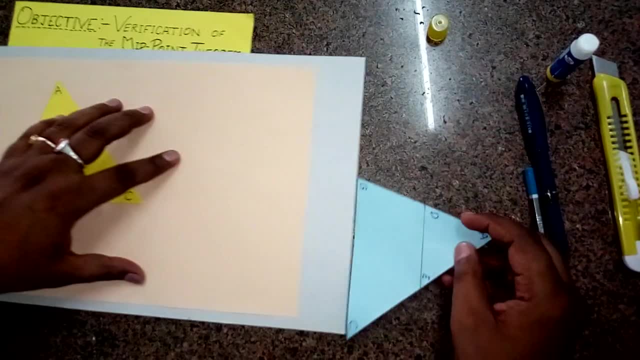 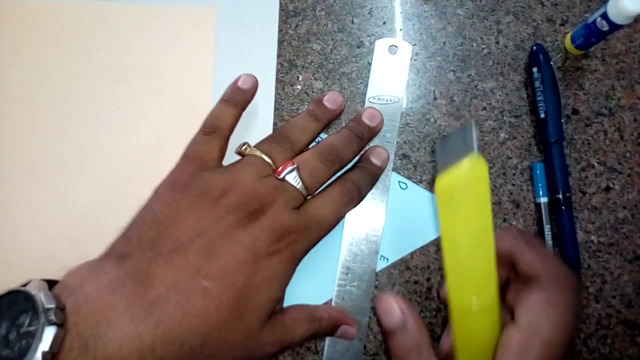 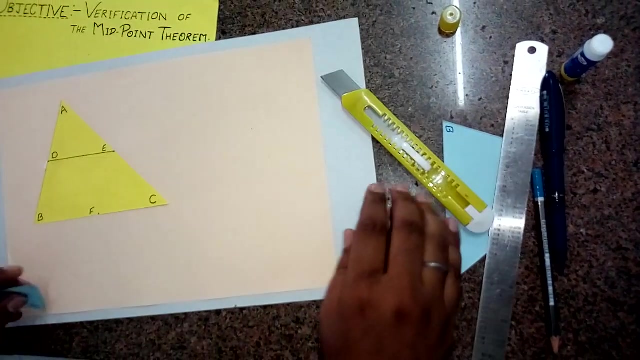 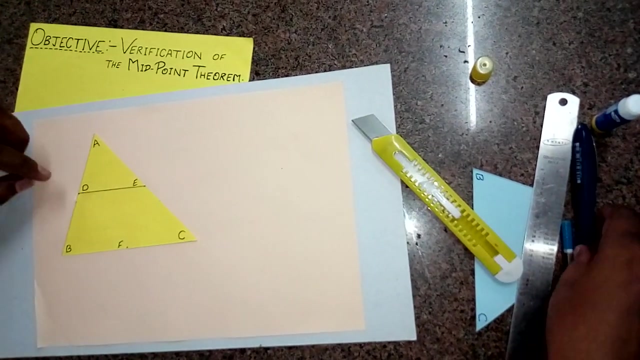 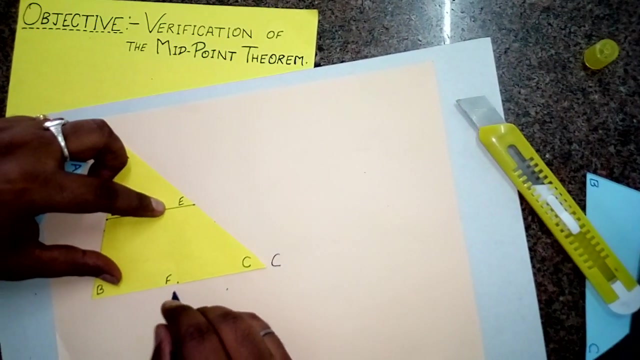 ADE. Now I am going to cut the triangle ADE along the line segment DE, So I am going to put it in a way that the angle E coincide with angle C. Now watch carefully, Since this one is C approval. I think it will hide behind it, So I am writing the point C over. 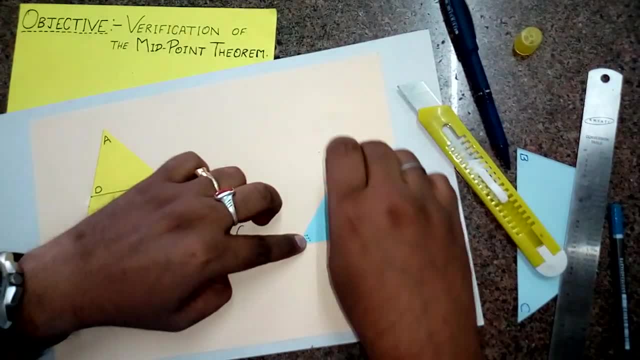 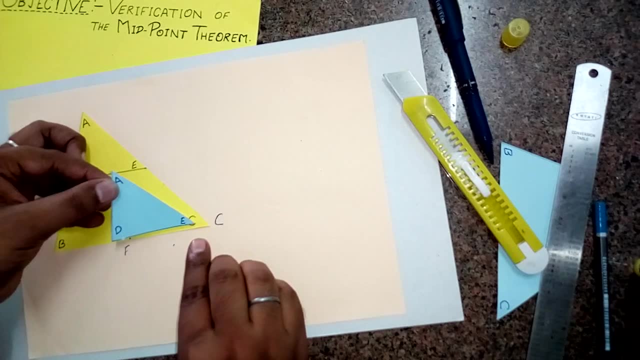 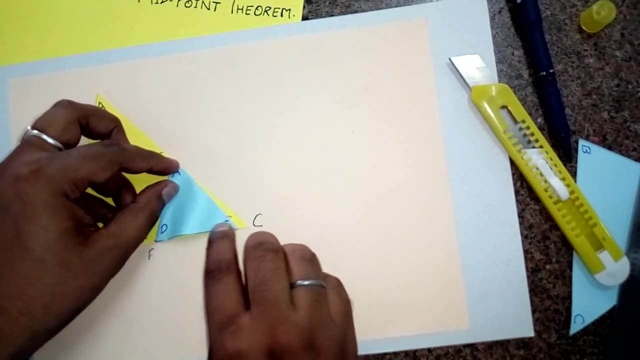 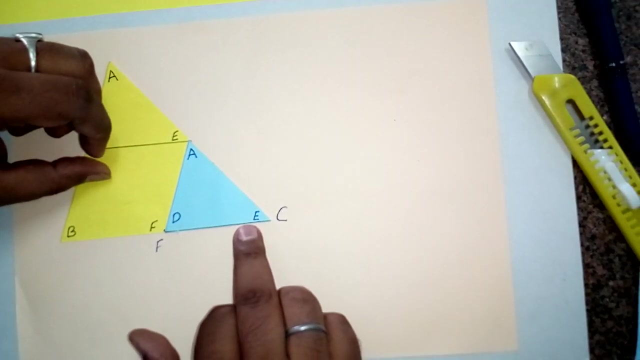 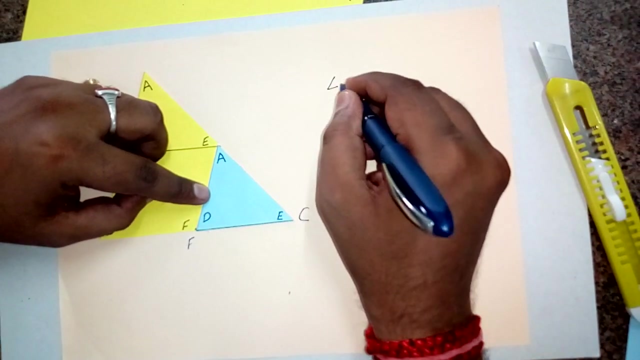 here, point F over. here We have to arrange it such that this E diagonal- will be the crystal of elimination- overlaps with C. Now, as you can see that this angle E had exactly overlapped the angle C, It means angle E and angle C are equal. So you can write that angle E is equal to angle C. 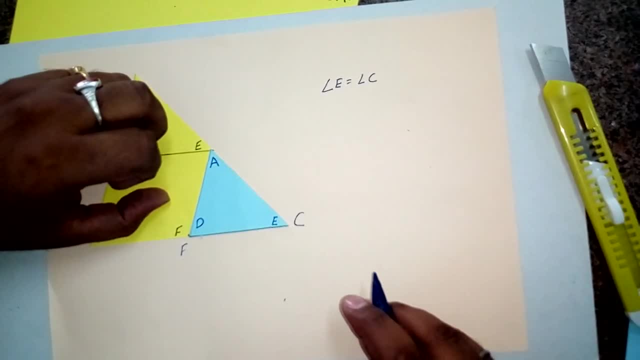 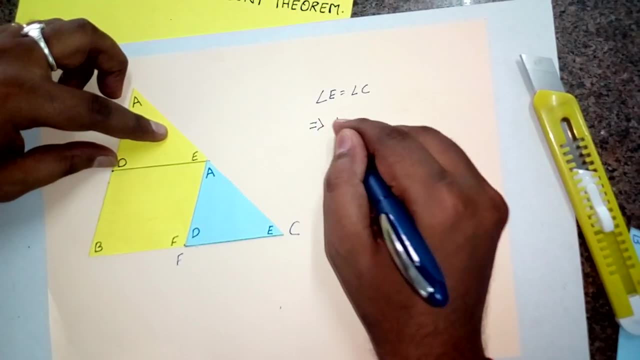 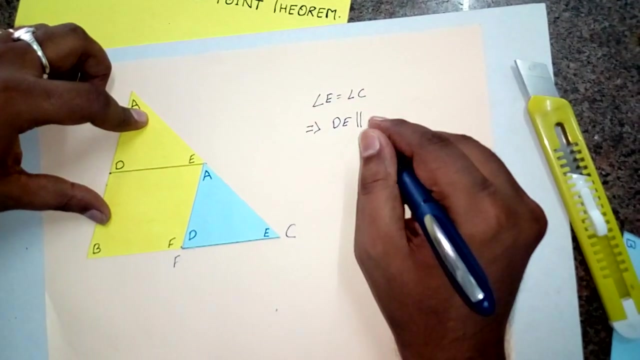 And these two angles are what Corresponding angles, And as the corresponding angles are equal, So the lines will be parallel. So this will imply this line DE, the angle E is parallel to the line BC, which contains the line C. So DE is parallel to BC. Our first part is proved. Now coming to the second part. 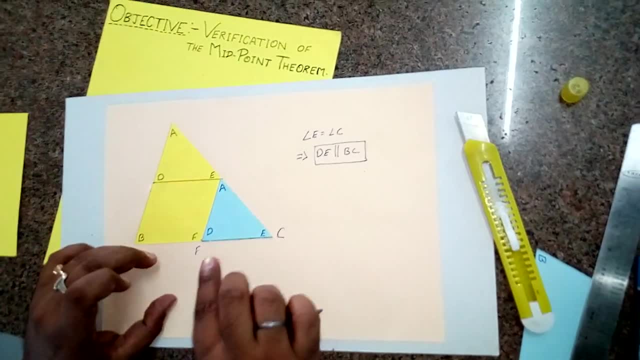 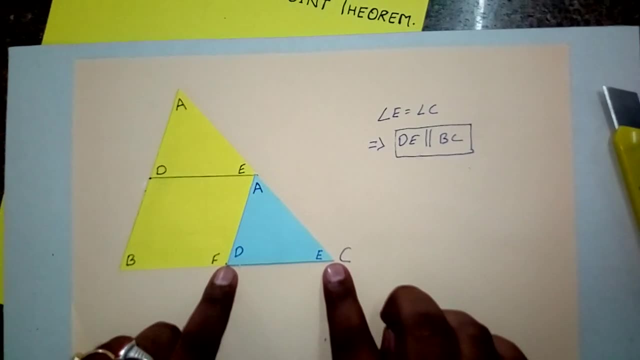 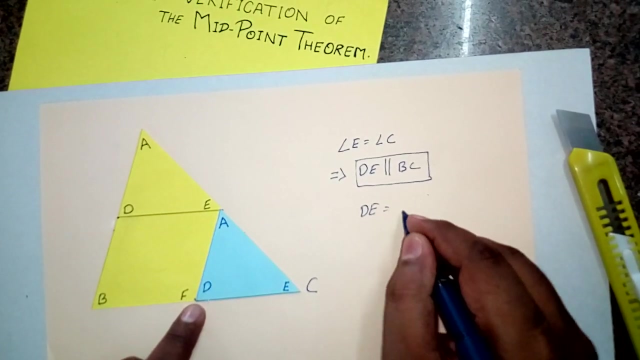 That DE will be half of BC. Now you can observe that we have got the midpoint F Of the side BC And DC is overlapping exactly that half portion of BC. That DE is equal to FC And FC was what The half of BC. 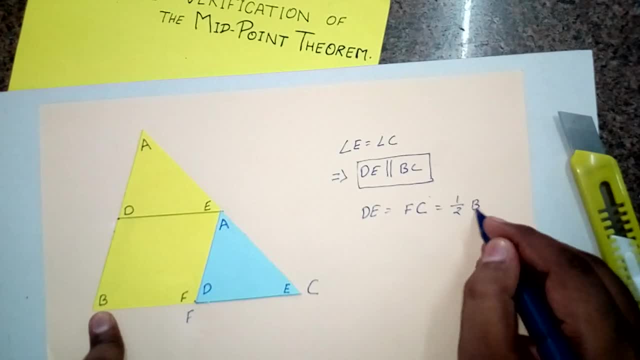 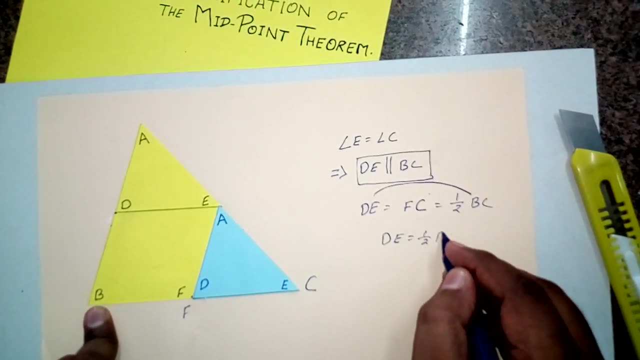 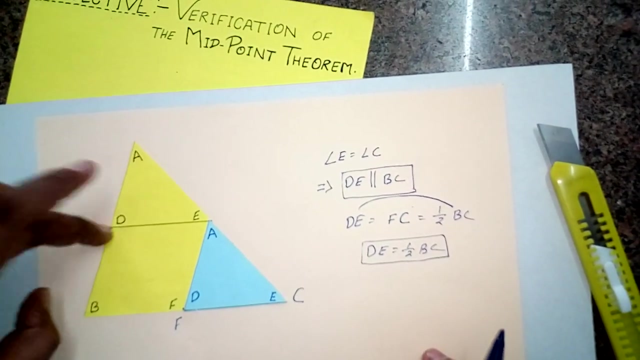 So in place of FC we can write half BC. So we can see that DE is half of BC. So DE is half of BC. So in this way I proved the Theorem that the line segment DE, joining the midpoints of two sides of a triangle, ABC, is half of the third side and parallel to the third side. 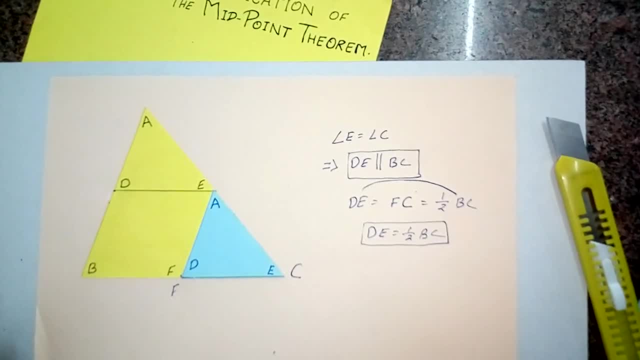 I hope you have learnt and you will be able to verify the theorem by your own. Thank you. 🎵.